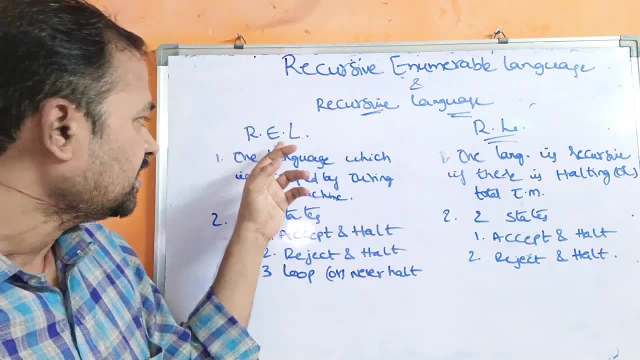 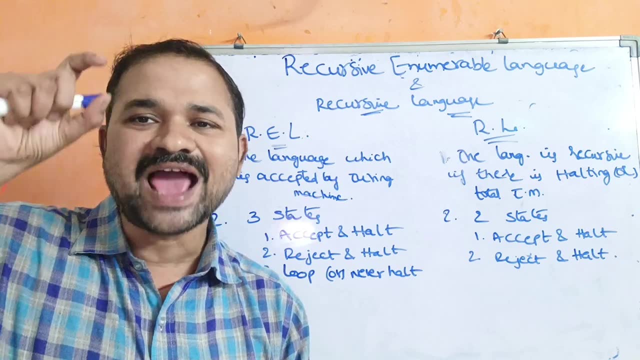 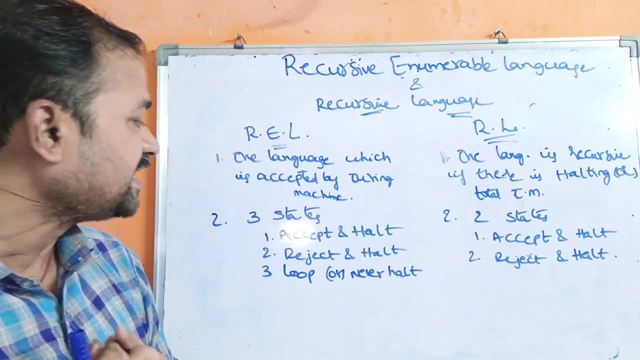 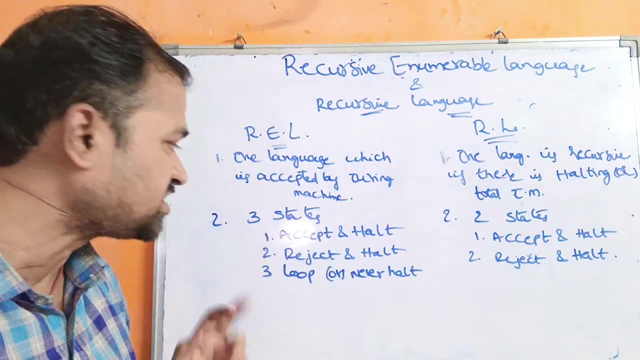 pushdown automata. So likewise here REL stands for recursive enumerable language. Recursive enumerable language means the language which is accepted by Turing machine. So the language which is accepted by Turing machine is called as recursive enumerable language. Recursive enumerable language mainly protects uses one of these three states. The first state is accept and halt. Second state is 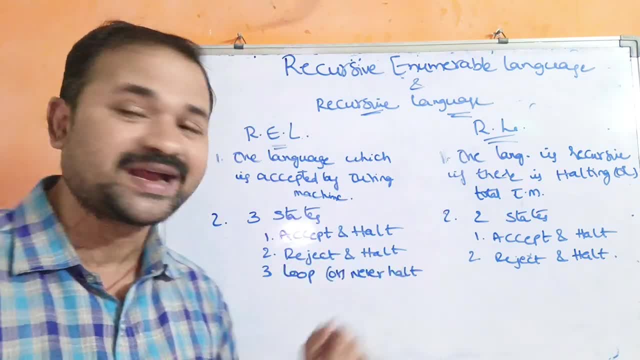 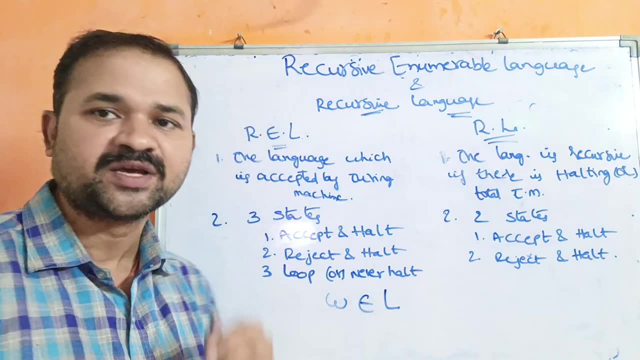 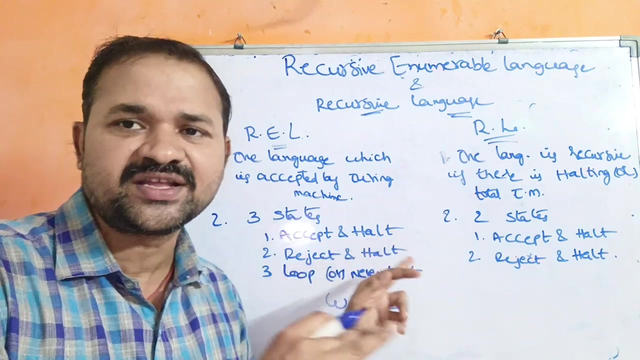 reject and halt. Part one is loop or never halt. So let us assume that we have a string W. If W belongs to the language, then we can say that the string is accepted by the Turing machine and after that it will halt. Suppose if the string doesn't belong to the language. 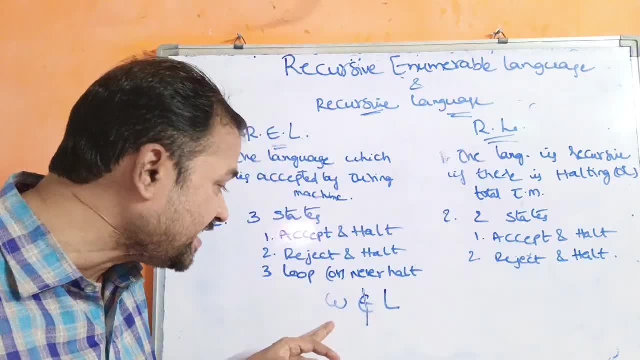 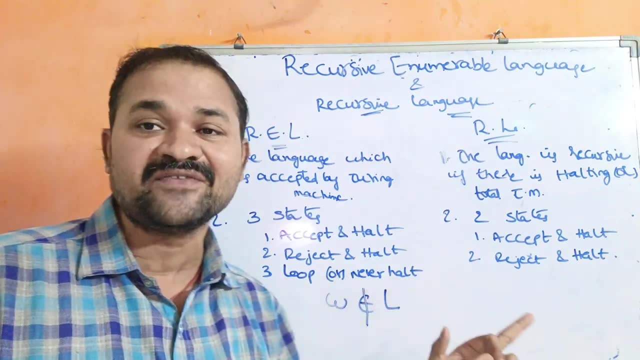 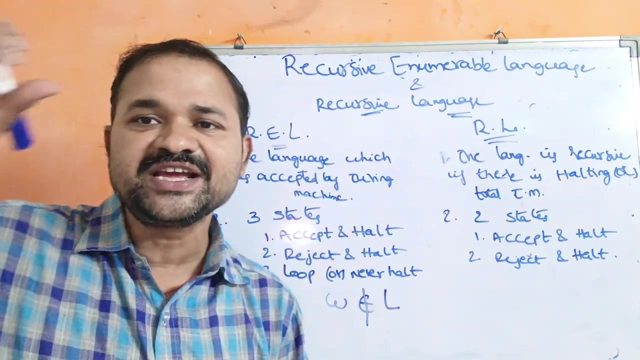 then we can say that the string is accepted by the Turing machine and after that it will halt. And one more scenario is loop or never halt. That means it never accepts nor resets if the string doesn't accept by the Turing machine, as well as if the string doesn't rejected by the Turing. 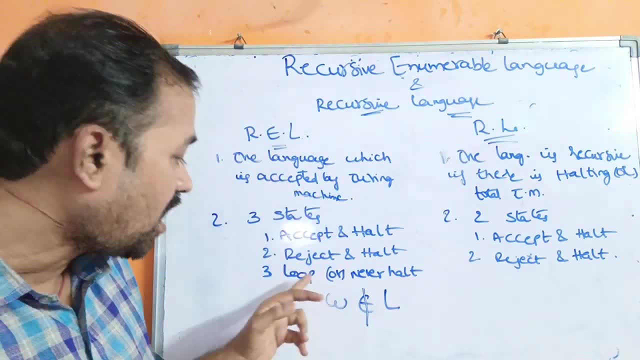 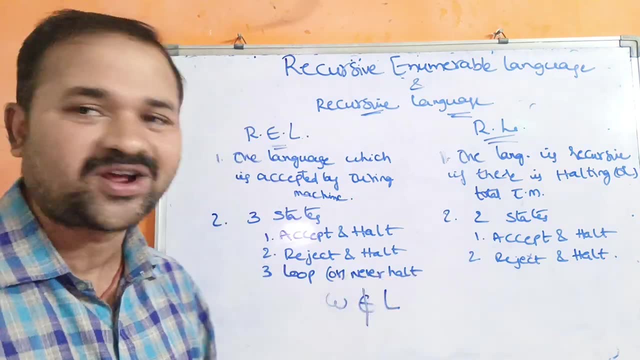 machine. Then it is called as what Loop state. So this is nothing, but here it will go into the infinite loop state. So this is nothing, but here it will go into the infinite loop state. So this state can also be called as never halt. So loop means neither accept nor reject. 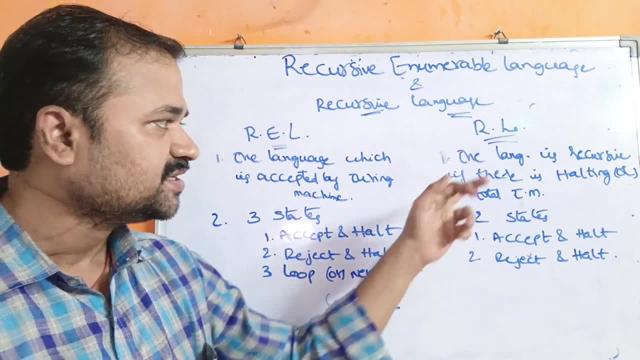 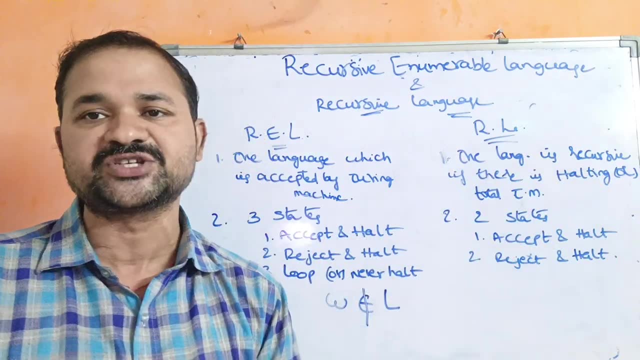 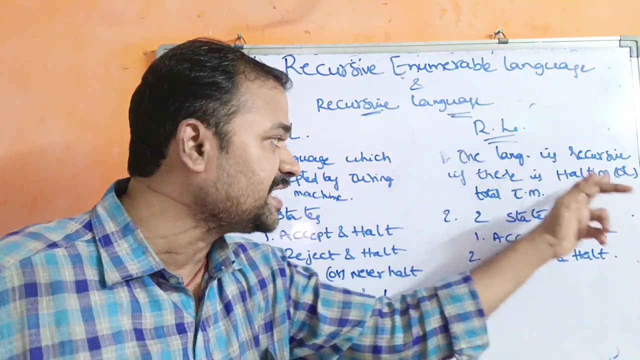 Now let us see about recursive language. The language, which is the language, is recursive if there is halting or total Turing machine. So we can say that a language is a recursive language if there is halting Turing machine or total Turing machine. So halting Turing machine or 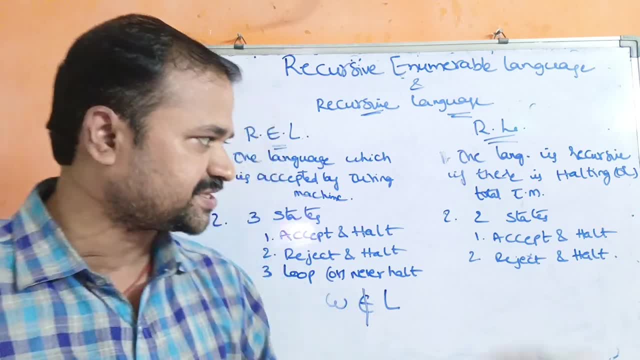 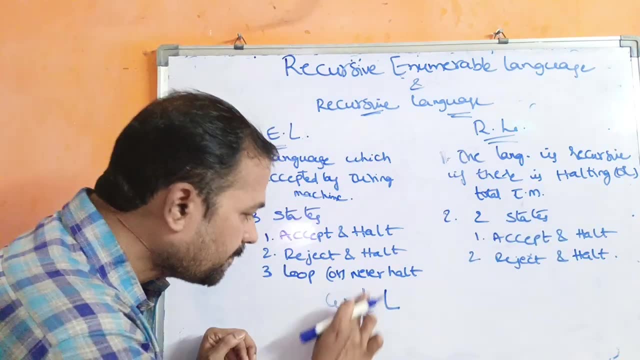 total Turing machine is a recursive language. if there is halting Turing machine or total Turing machine means it will produce only two states. The first state is halt and accept. The second state is halt and reject. Suppose if the string belongs to the language, then we can say that it. is accepted by the Turing machine. Suppose, if the string doesn't belong to the language, then we can say that the corresponding string is rejected by the Turing machine. So this is the major difference between recursive enumerable language and recursive language. In recursive enumerable language we may have loop also. Loop, or this can also be called as never halt, Whereas recursive language. 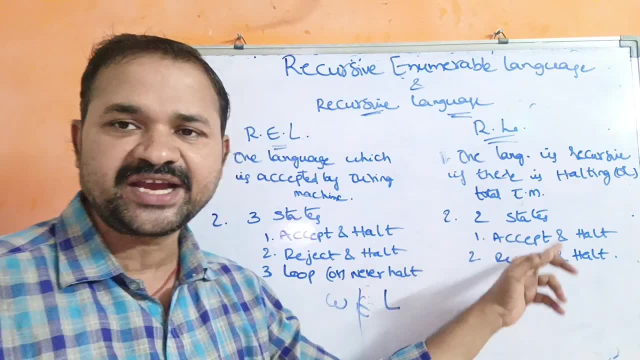 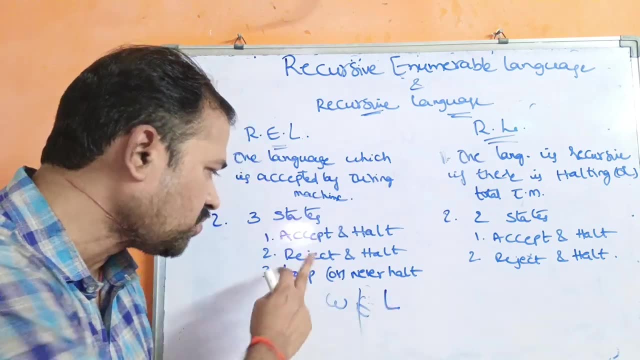 means. here we have only two states: Accept state or reject state, Whereas in recursive enumerable language in addition to the accept and reject we may have loop or never, halt also.